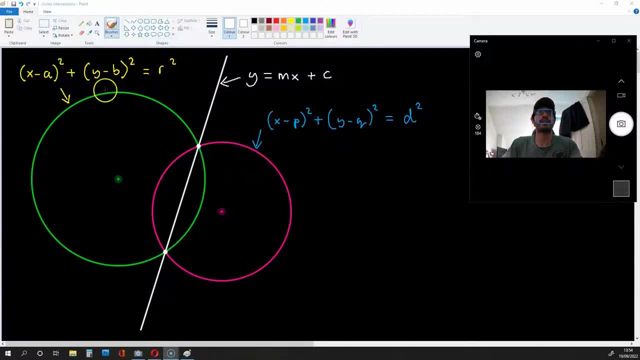 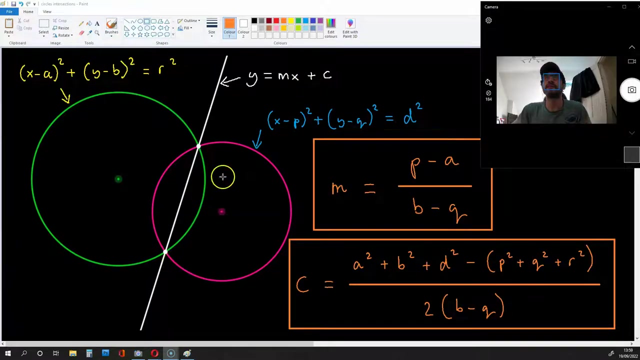 The equation of the first circle Is this, and the equation of the second circle is this: They have different centers and different radiuses, and the line cutting through their intersections is of the form Y equals MX plus C. Now, under these circumstances, for the line, Y equals MX plus C. 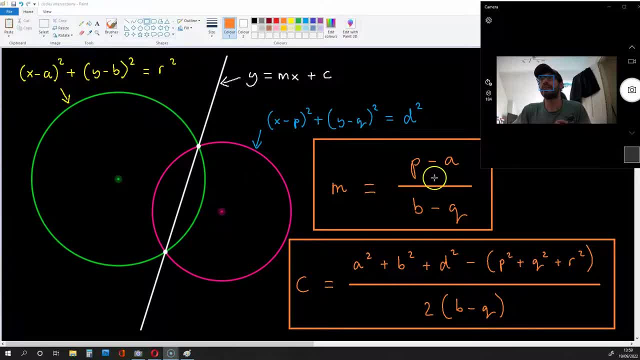 M is going to have the value P minus C Minus A, Over B minus Q, And C is going to have this long value right over here. If you'd like to know why, for this line, M is equal to this and C is equal to this? 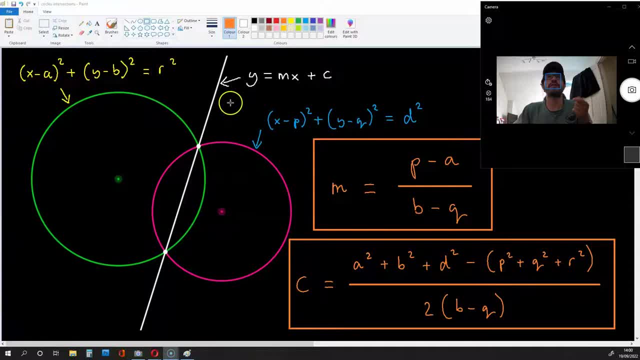 Then watch my previous video about how to derive the line that cuts through the intersection of two different circles. I've left the link to that video just below this one, So click on that link if you'd like to watch the video and find out how this line is derived. 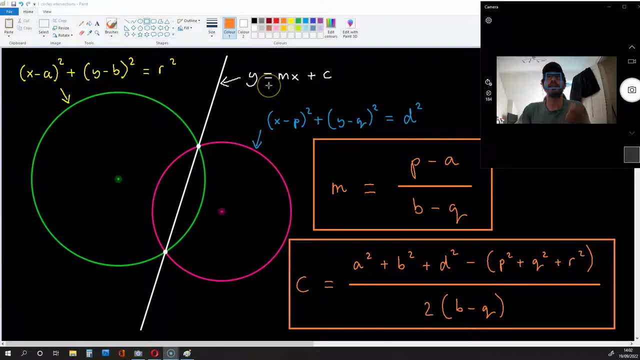 OK, so we know what this line is And we know where it cuts the green circle. OK, so if we plug this value of Y into this equation over here to the left, What we can get is a quadratic equation which gives us the X coordinates of these intersections right over here. 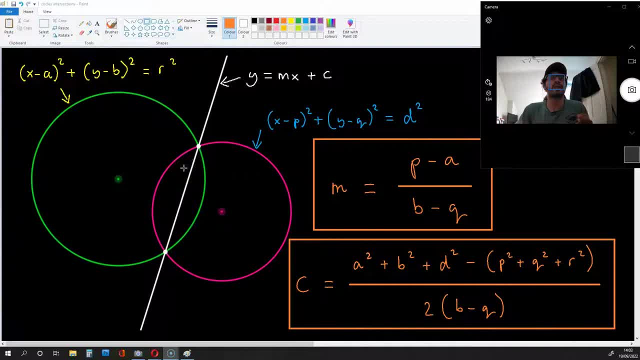 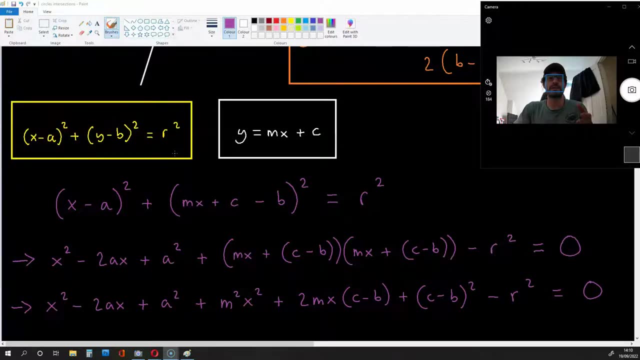 Once we have these X coordinates, we can find the Y coordinates. OK, and we have the complete coordinates of these two intersections over here. So we're now looking for the intersection points of the two intersections. We have this equation here, which is the equation of one of the circles. 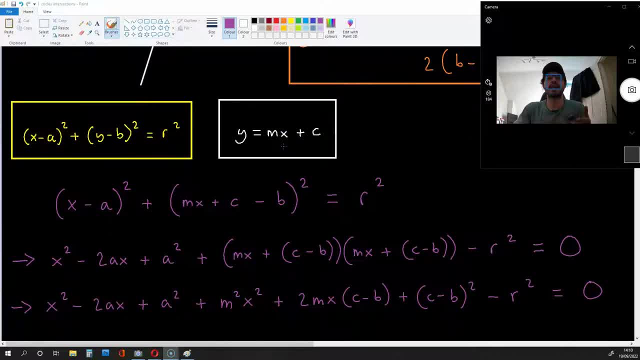 And we also have the equation of the line which cuts through the intersections. Now, if we replace the Y in here with MX plus C, What we can get is a quadratic equation for X Which gives us the X coordinates. OK, let's give this a go then. 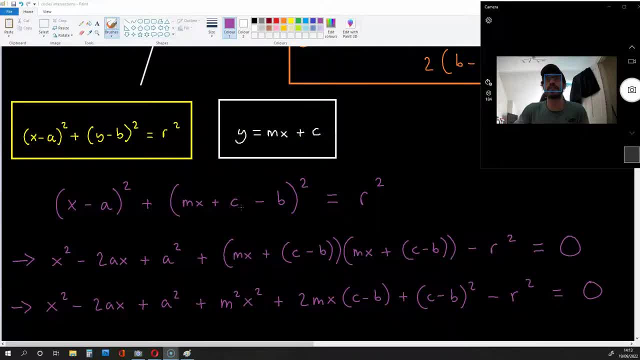 If we do that, we get this equation over here. And if we expand and send R squared to the other side of the equation, we get this. And if we expand further, we get this equation over here below And from here we can get the quadratic equation for X. 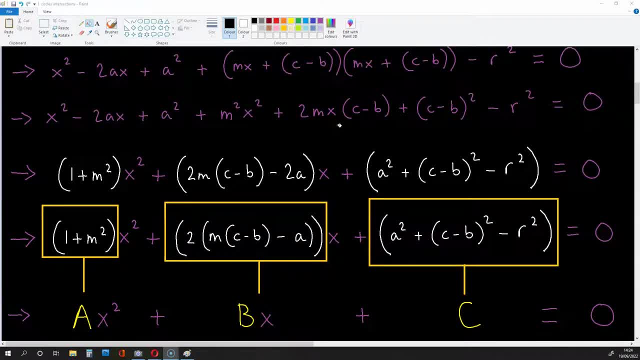 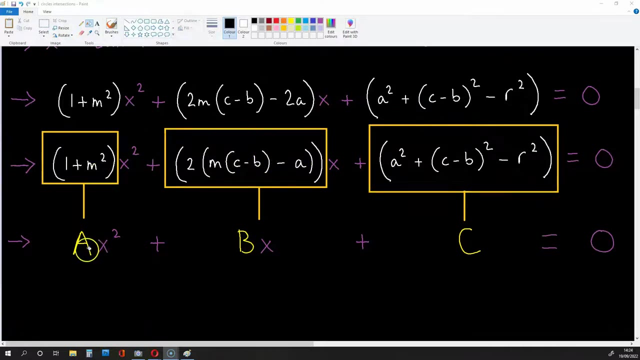 OK, so we want to be in the position where we can form a quadratic equation. So what we do from here is collect the coefficients And from here we get this equation over here, And these coefficients, OK, can be regarded as A, B and C. 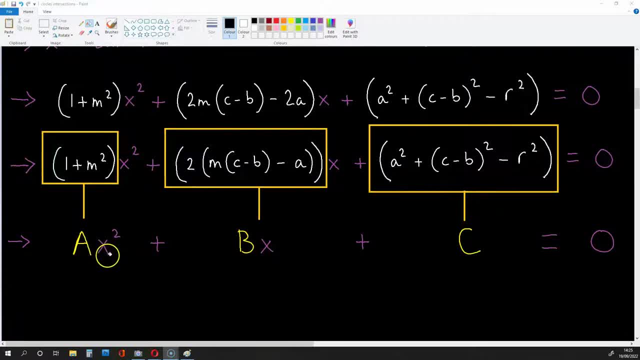 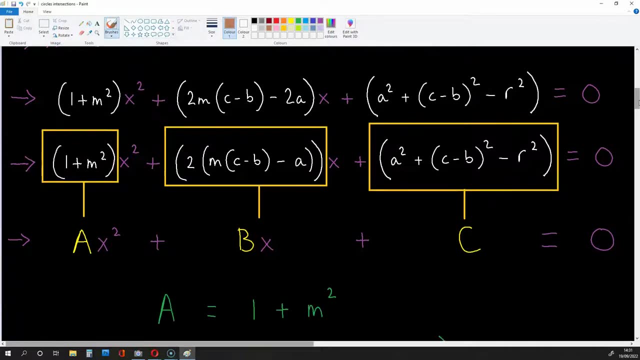 And if we have the equation right here And if we have the equation right over here, AX squared plus BX plus C is equal to zero. We can get the value of X for those intersections. OK, we're going to get the X coordinates of the intersections. 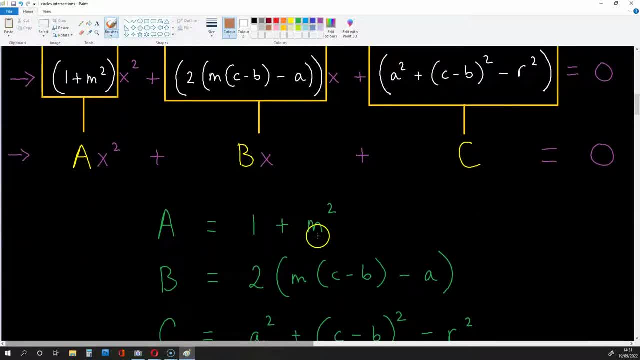 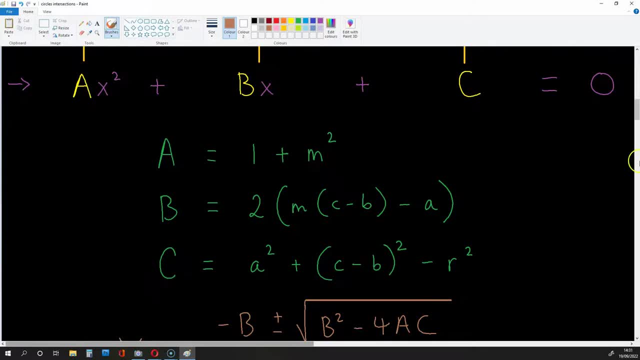 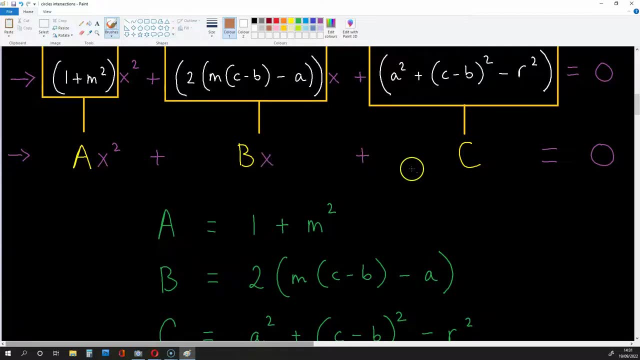 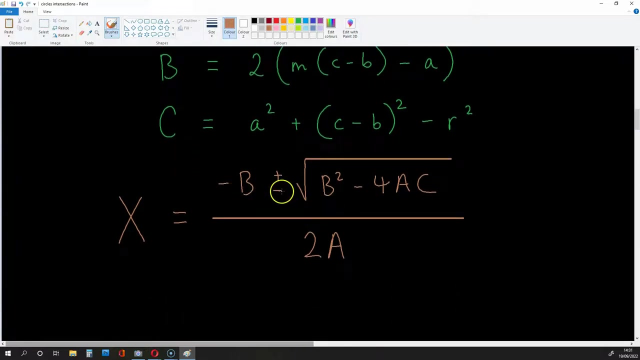 If we say that large A is one plus M squared, Large B is this And large C is this, From this equation over here, AX squared plus BX plus C is equal to zero. We get this value of X Minus B, plus or minus the square root of B squared minus 4AC over 2A. 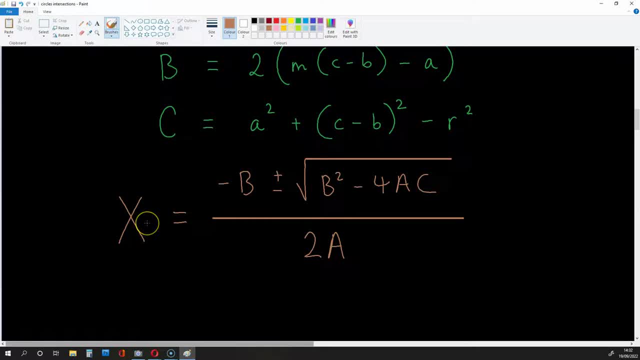 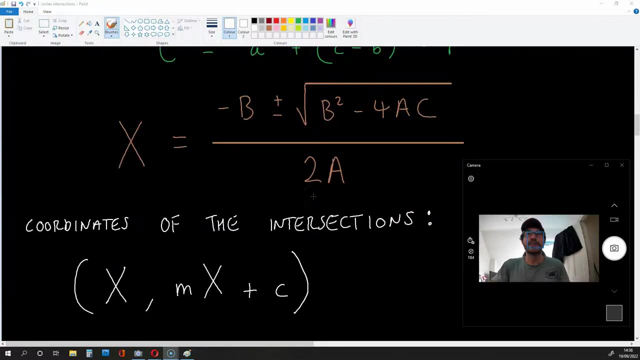 OK, let's call this value large X, Because we can plug this in To Y equals MX plus C To get the Y coordinates of the intersections. I know there's a lot of compression going on, But ultimately with this value of large X here. 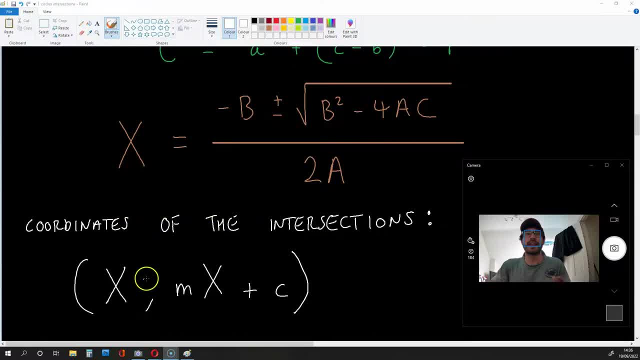 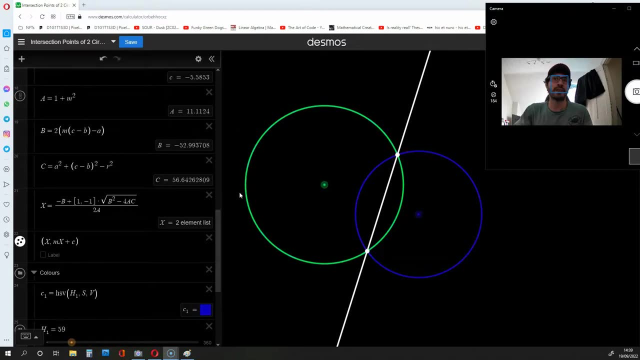 We get the coordinates of the intersections. That is, large X for X And M times large X plus C for Y. Now the best place to test out these equations is on Desmos. okay, So the value of large A can be seen over here, along with large B, large C, okay.